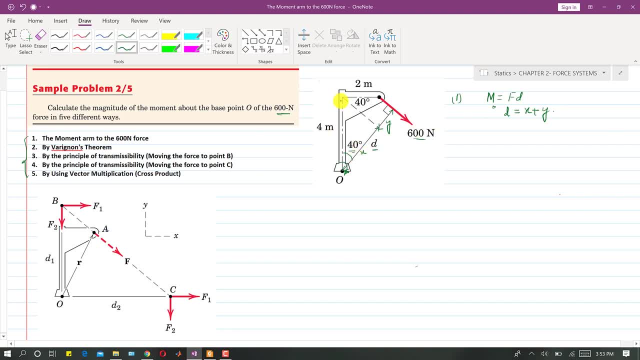 This angle is given, this angle is 40 and this length is 4 meter. So if, let's suppose, if I consider this O AB triangle, This point is B. So if I consider triangle O AB, So then X is equal to 4.. 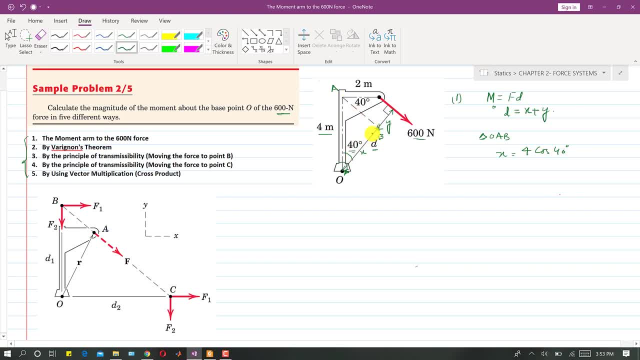 Cos of 40 degrees right. So in this O AB triangle this X is the base and 4 meter is the hypotenuse. So X is 4 cos of 40 right. And now in here, If I draw another parallel line to this Y length. 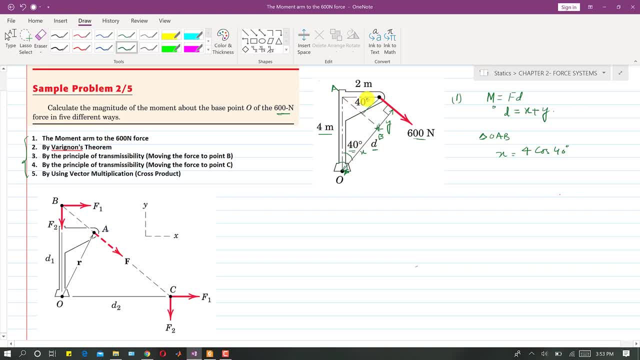 So then we have this triangle right And in the problem, it is given that this force is making 40 degree with the horizontal right. So if this line, if this line is parallel with this force, so then if this is 40, so then this angle is also 40, right? 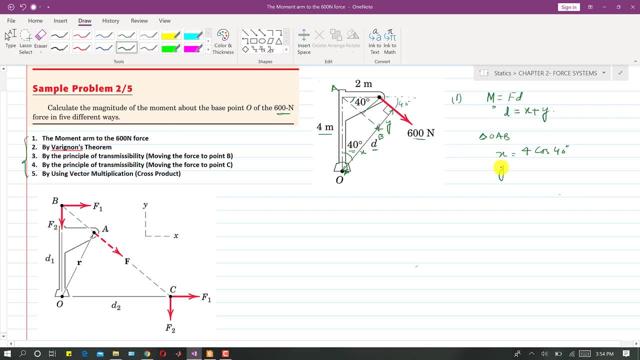 So this means that Y length is equal to. if this is the hypotenuse right, So then this is the base And this is the perpendicular. If this is 40. So then this means that this will be 2 sin of 40 degrees, right. 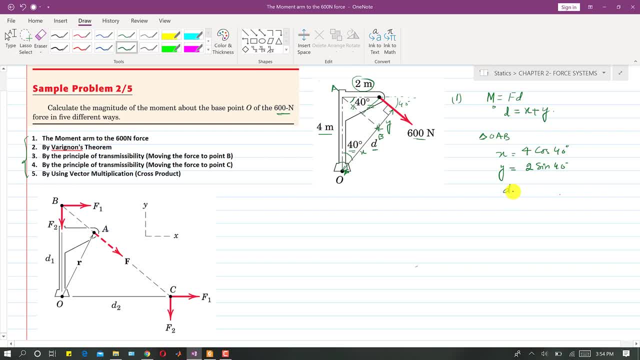 So then, what will be? D So D? the perpendicular distance of the force from the point of rotation, from the axis of rotation, is D, Which is X plus Y, So it is 4 cos of 40 degrees plus 2 sin of 40 degrees, right? 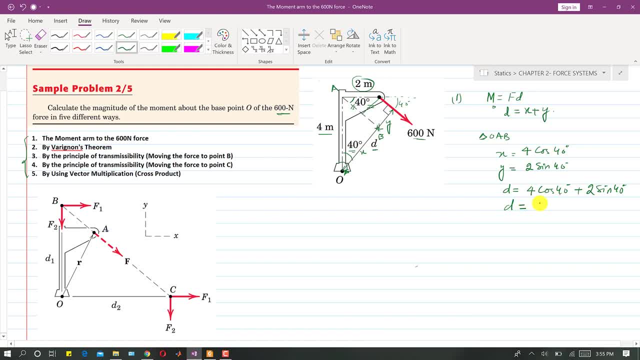 So then D equals to 4.35 meters. So this is the perpendicular distance of this force: 600 Newton. So then we can find moment about O. So then moment about O. Let me write it here. So moment about O will be equal to F. 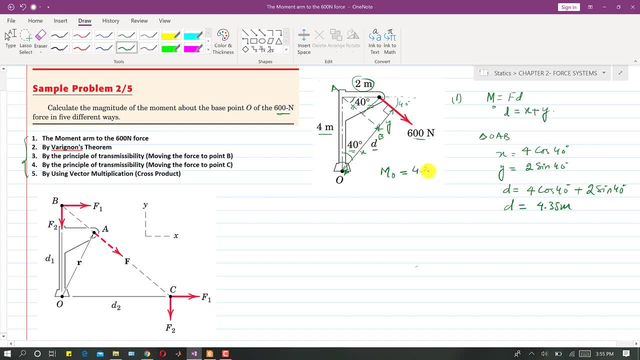 So F is how much? F is 4.35 meters Into 600.. Right, So then this equals to 2610 Newton meters. Right, So this equals to 2610 Newton meters. And if we use right hand rule, So the direction is towards the page or the screen right. 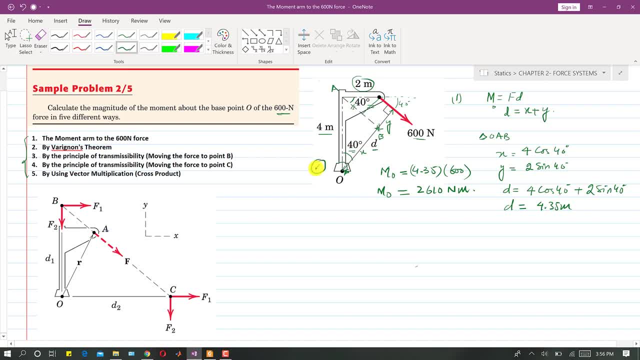 So this is the direction. The direction of the moment is towards the screen, So we can write it here as clockwise And this is the direction right. So this is using This is the value of moment, using the first method, The second method. 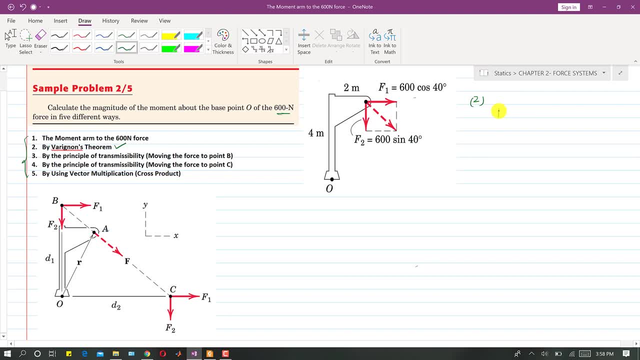 And this is using the Waring-Nag's theorem. So Waring-Nag's theorem said that The moment of a force Is equal to the summation of moment Of its components, Right? So this means that the summation of the moment of F1.. 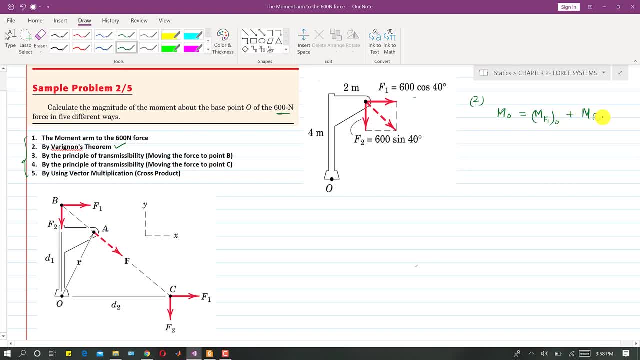 About O plus the moment of F2.. About O Will be equal to the total moment of the 600 Newton force. So this means that if we resolve this 600 Newton force Into its components And then we find the moments of individual components, 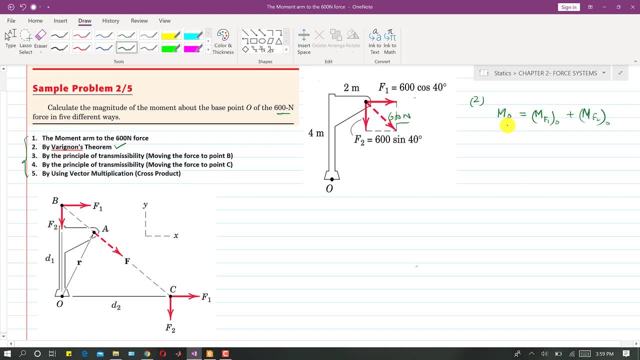 And then we take the sum of those components, So that will be equal to the total moment Of that force, right? So this is Waring-Nag's theorem. So now, If this is 40. This angle is given, This is 40 degrees. 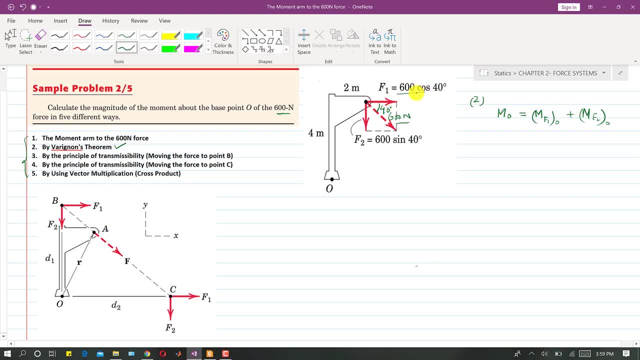 So if this is 40. So then this component, This component is 600 cos of 40. And this component is 600 sin of 40.. Right, So now, This length, This length is that distance D, Which is making 90 degrees. 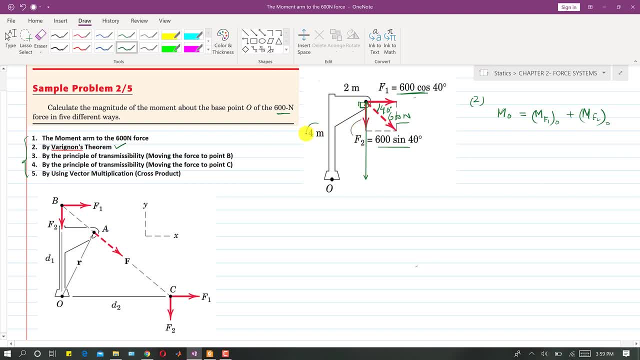 So this length, This means that this 4 meter length Is the perpendicular distance of this F1. From this point of rotation. So this means that if I write Moment about O, So, then this will be equal to So for. 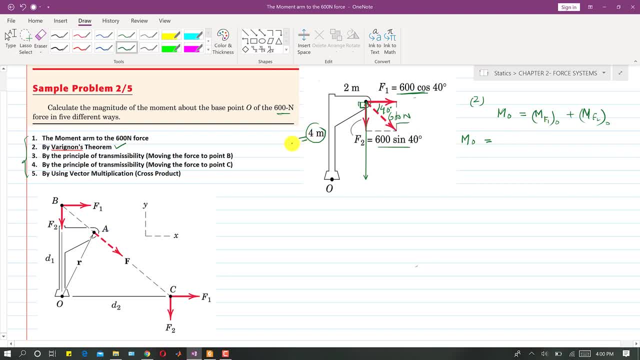 Let's suppose for F1. This distance is, let's suppose, D1 right And the perpendicular distance of the F2 force, This force, This is the distance for the F2.. So let's suppose this is D2 right. So this D2 is the perpendicular distance of this F2.. 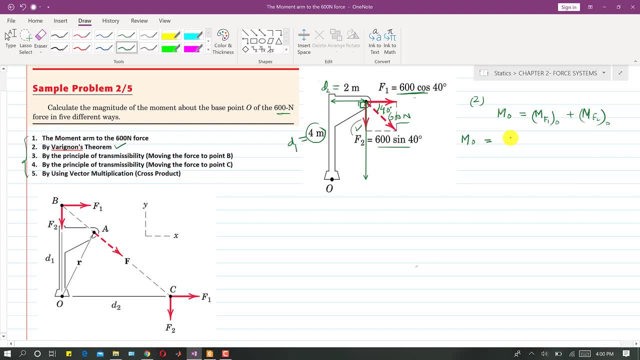 From the point of rotation, right? So then this will be F1. Into D Plus F2.. F1 into D1. And F2 into D2, right? So then F1 is what? F1 is the 600 cos of 40.. 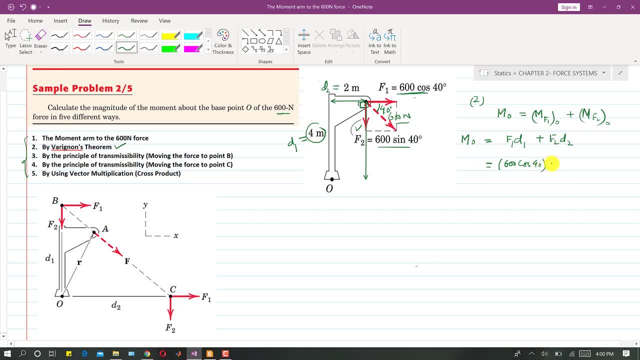 It's the component of the 600 Newton force Right, And D1 is how much D1 is 4. Plus F2. So F2 is how much 600 sin of 40 degrees into D2. So D2 is 2 meters. 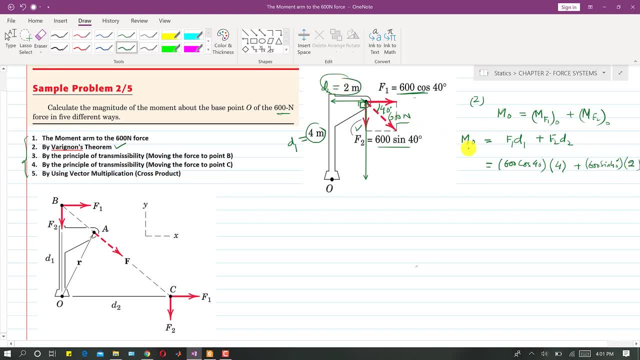 It is given. So this distance, This is D2.. So if we calculate Moment about this point, So again it will be equal to 2610 Newton meter. So by applying We get the same moment For this 600 Newton force. 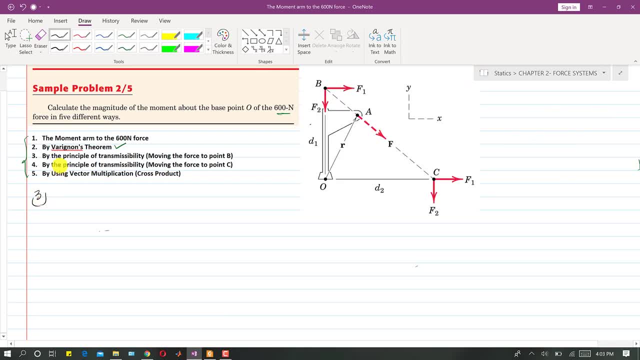 Now the third method Is that, By the principle of transmissibility, Moving the force to point B. So if the Principle of transmissibility says that We can move this force Along its Line of action As long as its resultant is not affected, 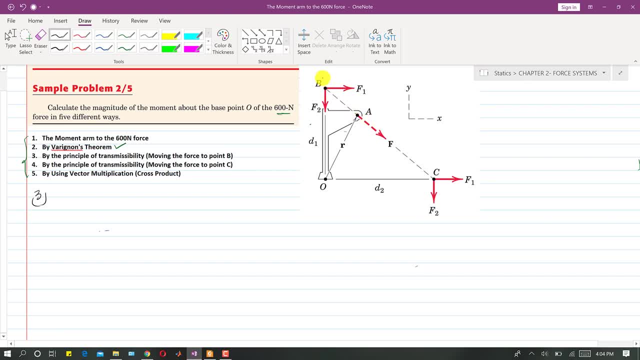 Right. So if we move this force to this point B, If we move this force to this point B, So then If we find the moment of this force, So then The F2 component, The moment produced by F2 component, will become 0.. 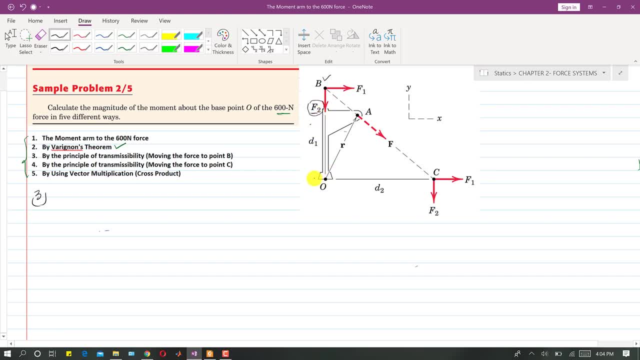 Why? Because this F2 force is passing Through this point of rotation, Through this axis of rotation. If it passes through the axis of rotation, Then it will never produce the Rotational effect, So they will not produce the torque. So in other words, 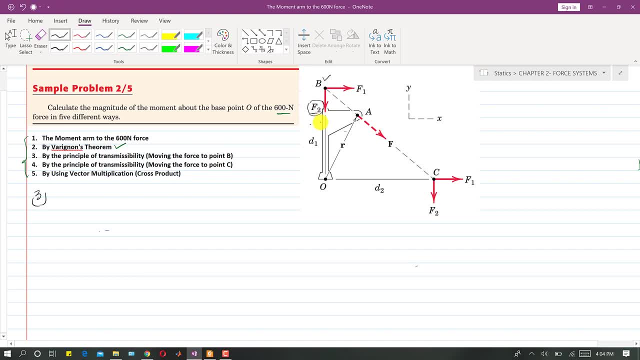 If the component, If the force is passing through the axis of rotation, So it will not produce any moment, Right? So here F2 is not producing any moment, Only the F1 component of this force Is able to produce The moment about this point O. 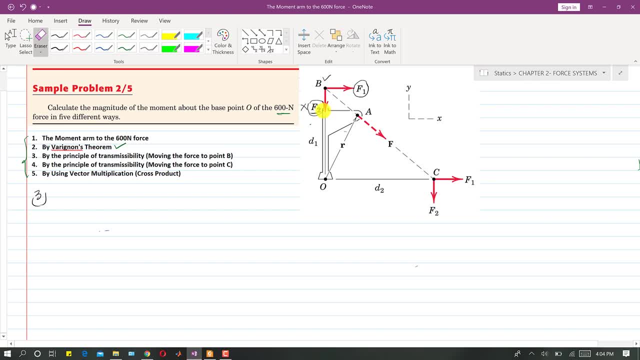 Right, We need to find the total Perpendicular distance of this F1. From the point of rotation. So now, if I draw A line here, Let's suppose if I draw This line, We need to find this distance, This distance. 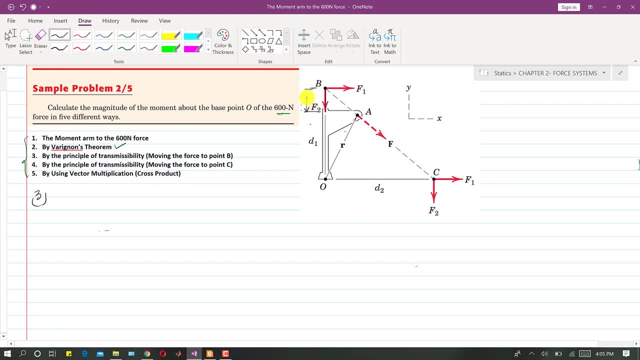 So we need to find this distance. So then we will be able to find The total distance of this F1. From the axis of rotation For this distance. So let's suppose if this distance is X, So then the total Distance of this force, 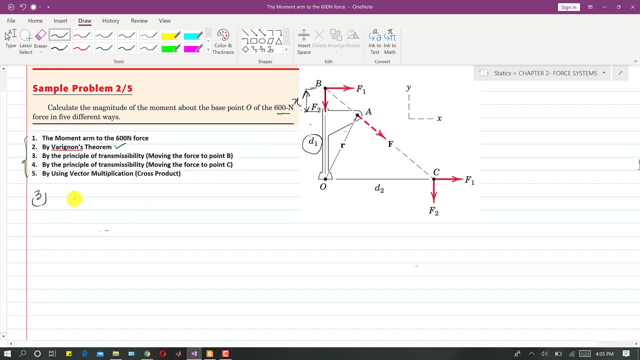 From the axis of rotation Will be how much So that distance will be? Let's suppose I write, The total distance will be D1 plus X. So now we need to find this X distance If this is 40 degrees. 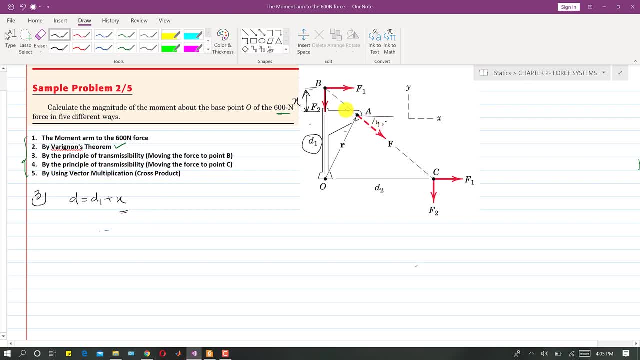 Right, This is given in the initial diagram. So if this is 40. These two angles are vertical angles And we also know that This length is 2 meters, Right? So then we need to find this X distance. So now, if I apply, 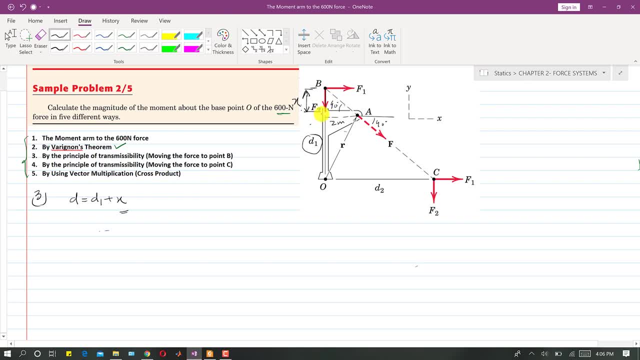 10-40 degree to this triangle. Let's suppose I write that Here. let's suppose we have this P point. Let's suppose so ABP triangle. So if I apply, If I say that triangle APB, If I apply, 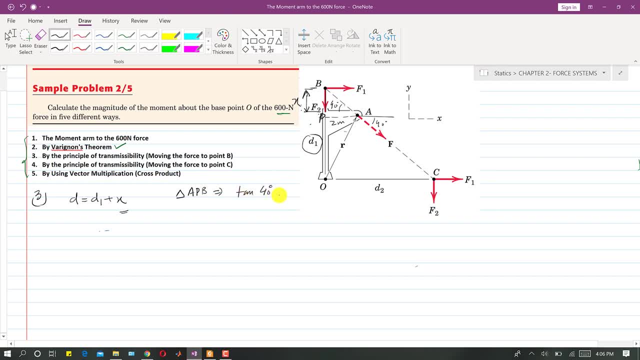 10-40 degrees, So then 10-40.. And the perpendicular for this Triangle is X. For this, theta is: For this: 40 degrees is X, the perpendicular, And the base is 2 meters Right. so then X is equal to. 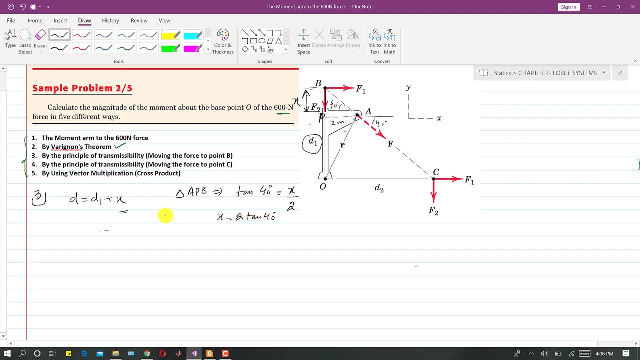 2-10-40 degrees, Right. So the perpendicular distance of this F1 component From the axis of rotation is this: D, D1 is 4. Plus 2-10-40 degrees, Right? So then, if you want to find the moment, 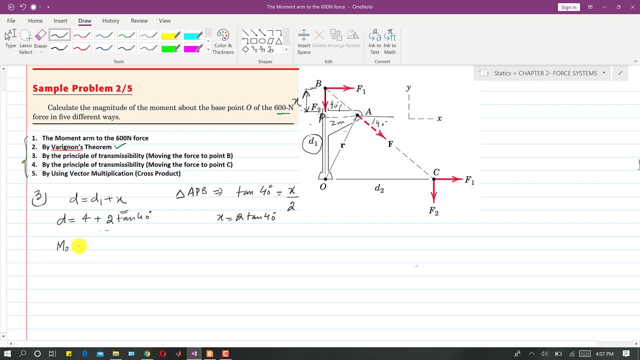 The total moment Of the force about point O. So then this will be equal to F2.. Into its perpendicular distance. Let's suppose that distance is. Let's suppose D1 right, And then F1.. Into D From zero right. 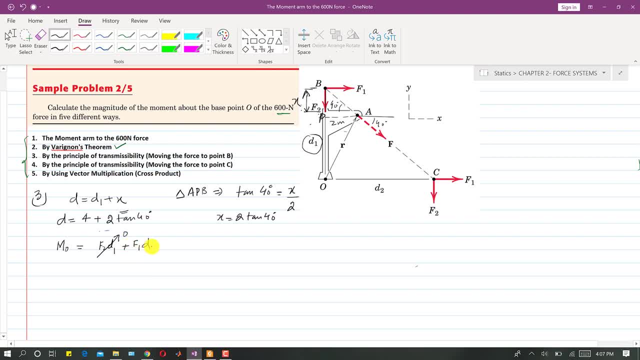 So we are only left with F1 and its perpendicular distance. So now, if I write So, F1 is how much? F1 is 600.. Cos of 40 degrees, It's the component of force along the X axis. 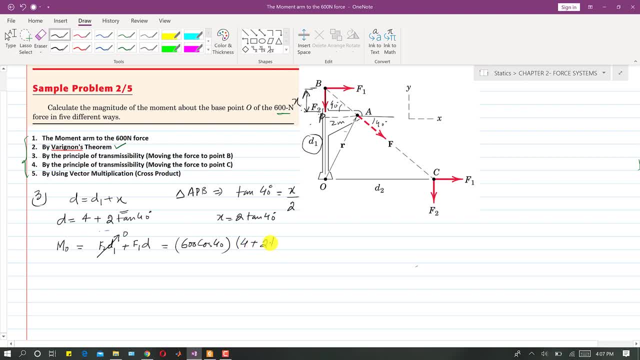 Right, and then we will write 4 plus 2. 10-40.. So now if we multiply this Using calculator, So what we will get Is the momentum: The same moment. Now we will use the fourth method, So the fourth method is again. 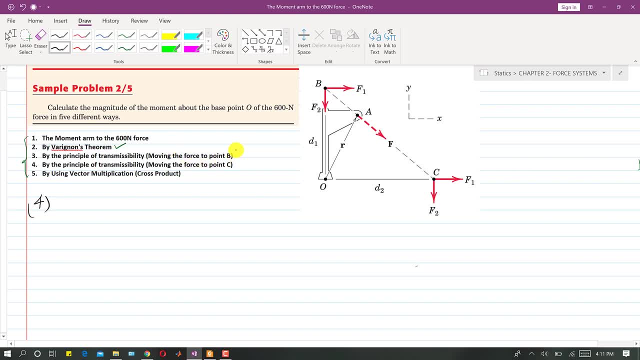 By the principle of transmissibility, Moving the force to point C. Now, if we move this force Along its action, Along its line of action, To this point C, So then we can find the moment as well, right. So now the F1 component. 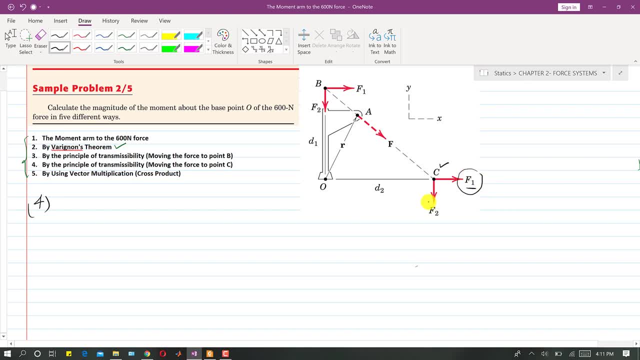 The moment produced by F1 component Will be equal to zero And the only component left Will be produced by this F2 right. So now we need to find this D2 distance, This D2 perpendicular distance Of this F2 from the axis of rotation. 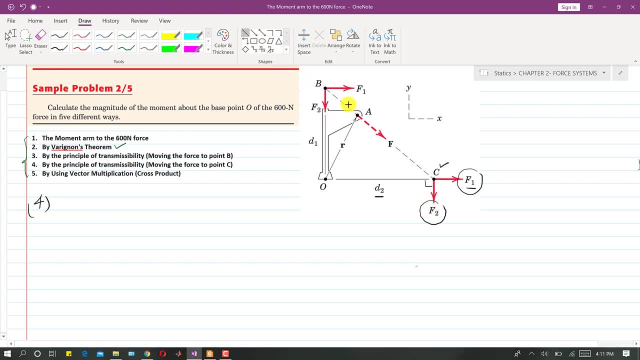 So let's suppose if I draw a triangle here, Let's suppose, Let's suppose if this is a triangle now, Let's suppose I write: this is D, right, So this A, D and C. So this is A, D and C. 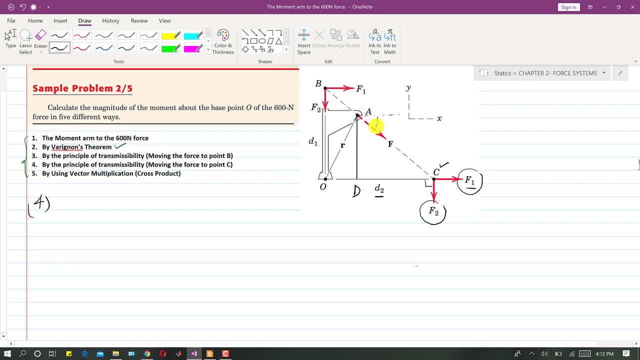 So if this angle is 40, which is given, So this angle is also 40 degrees. These two are alternate angles, right, This is also 40. And also, We have solved this triangle as well. We have solved this triangle. 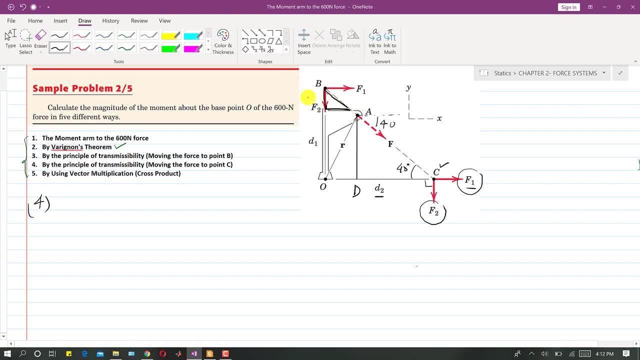 Just before, Just in the third method, right? So this was X distance And this distance was 2, 10,, 40 degrees, right? So we know this length And this length is 2, right? So, as we see here, 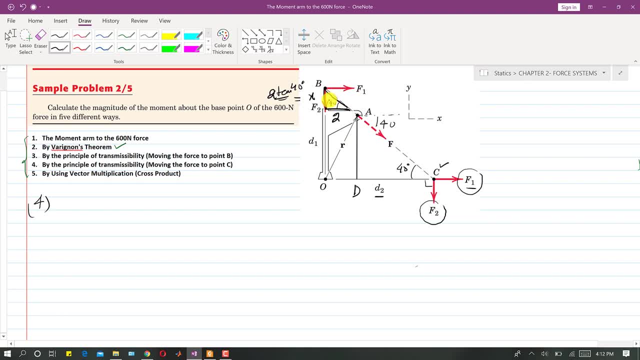 That this is also 40 degrees. So this small triangle And this triangle, this large triangle, Both of these are similar triangles. So for similar triangles, The ratio of the corresponding size Are equal. right, So now let's suppose if I write. 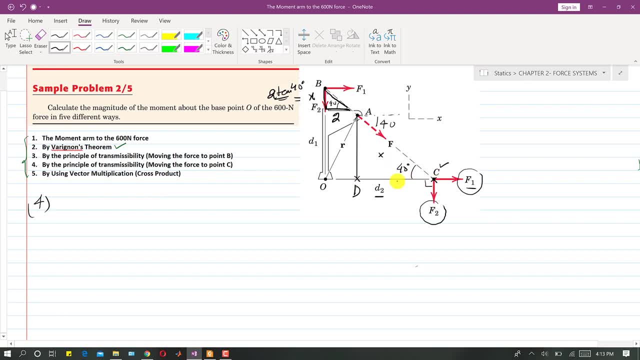 The distance from this point to this point, The DC distance. Let's suppose the DC Distance is Y right And the OD distance is How much? This OD distance is 2 meters, So D2.. The distance of F2.. 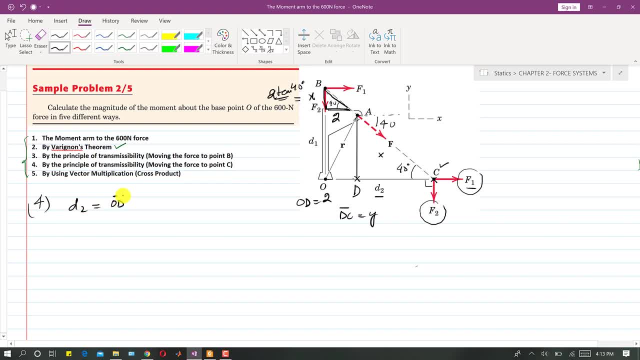 From the axis of rotation Will be equal to OD Plus DC, Which is Y right. So OD is 2. Plus Y. So now we need to find this Y. So now, if I write Y, This Y distance Divided by this AD distance, 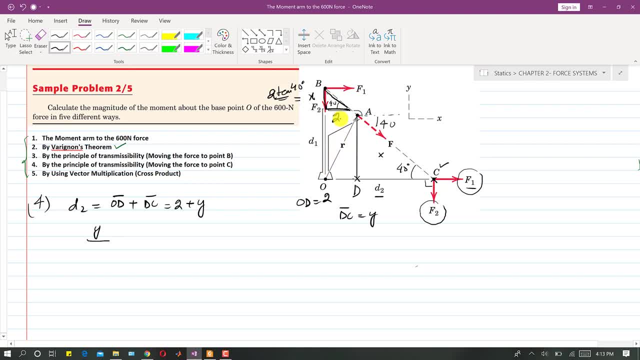 So AD distance is 4.. Which is given, So this AD distance is 4 meters Right. so this is given, So this is 4.. And now these two triangles Are similar triangles. So now, if I take the same ratio, 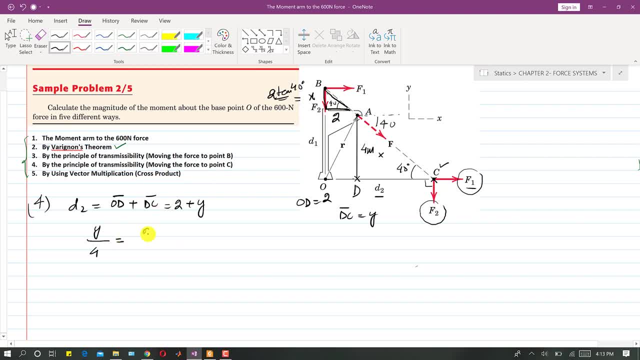 So that ratio will be equal. This will be 2.. Divided by X, Right, this perpendicular distance Right, this is Y Base divided by perpendicular. So, again, this will be base Divided by perpendicular, Y Divided by 4.. 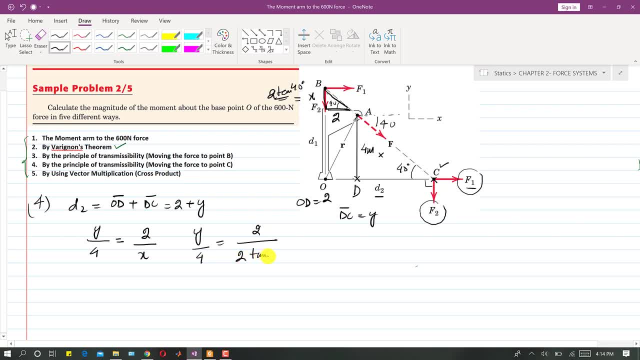 This will be equal to 2. And X is 2. 1040 degrees. right, So this will cancel out. So then, Y will be equal to 4. Divided by 10. 40 degrees. Or we can write it like this: 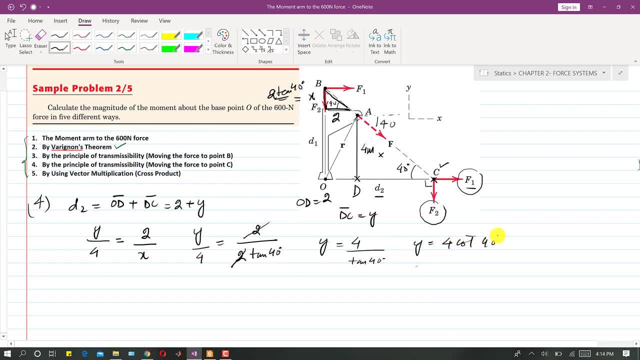 4. 40 degrees, right, So this is Y. So now D2.. So D2 will be equal to 2 plus Y. So what is Y? Y is 4 cot of 40 degrees. So now, if you find the moment about O, 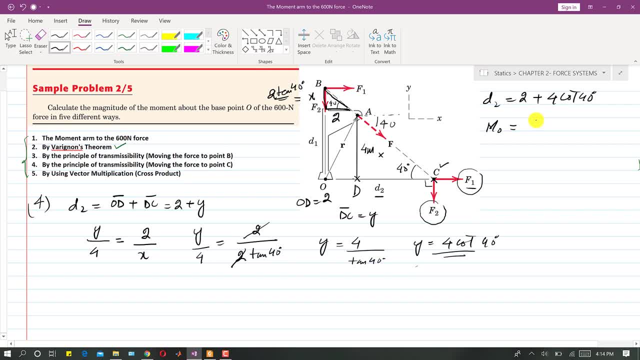 So then this moment will be equal to F into D, So now F2 into D2.. Right, So F2 is how much this F2.. So this F2 is the sine component, So this is 600.. Sine of 40 degrees. 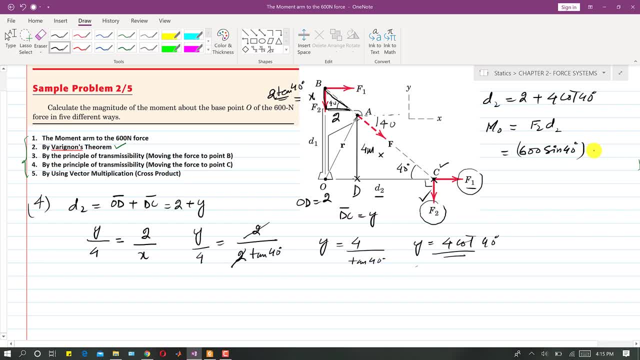 Right And into D2.. So 2 plus cot, 40 degrees. So now if we apply this, If we use calculator, So then again it will be equal to 2610 Newton meter. So this is the third method. 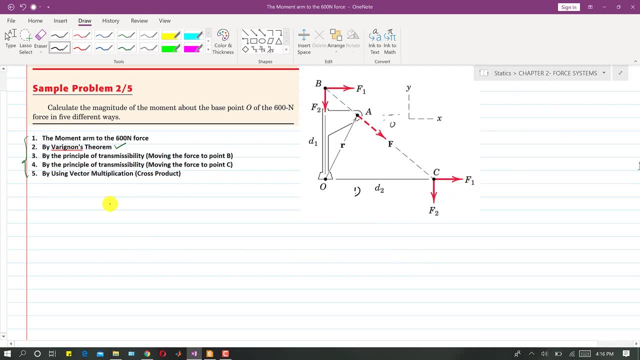 Sorry, the fourth method. Now the fifth method is that By using vector multiplication, That is the cross product. So we know that R cross F. So if we know The vectors of R and F, So then we will take the cross product. 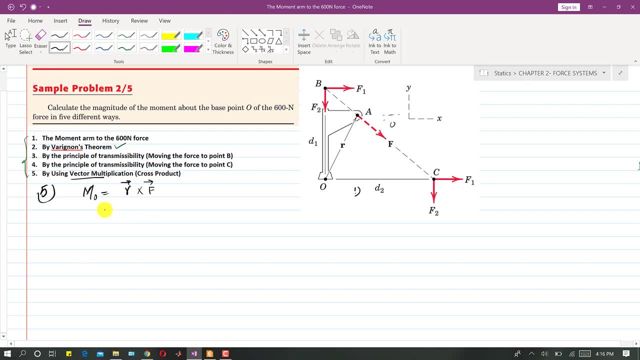 Of those vectors. So then we will get the moment about O. So this is R vector, Right, So this is OA is R vector. So the components of this R vector are what? So let's suppose, if I write, This is the one component of R. 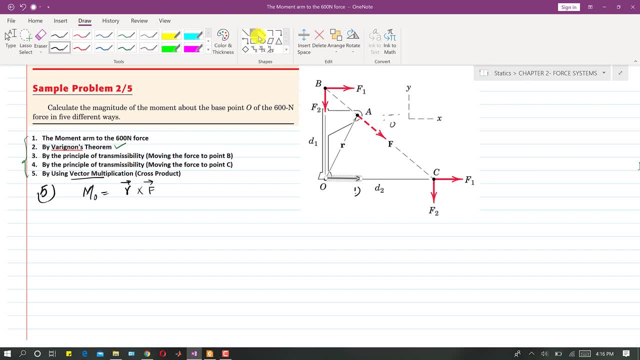 And This is the second component of R Right. So the length of this component Is 2 and this is along X, And this is 4 and this is along J Right. So if this is the positive X direction And this is the positive Y direction, 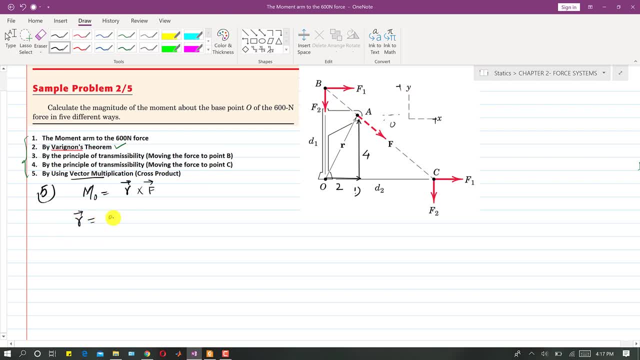 So then we can write: R vector Is 2i plus 4j, Right, So this is the R vector And already we have resolved, Resolved this force into its component. So if I again draw, This is the F1.. 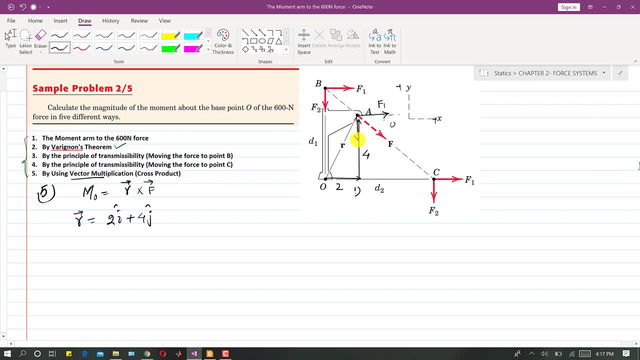 And Here this is the F2 component That we have already discussed here. So now the force vector Will be equal to F1i Minus F2j. This component is In the negative Y direction, So F1 is. 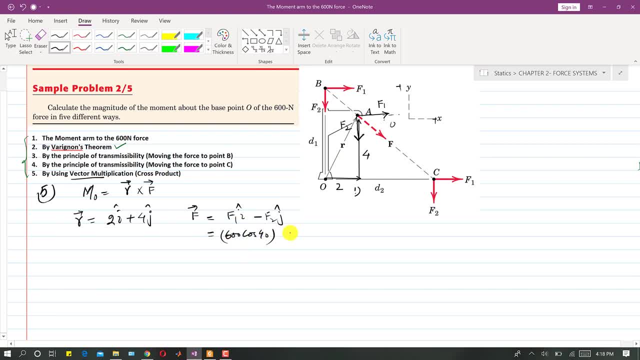 600 cos of 40 degrees I Minus F2 is 600 sin of 40 degrees Towards J Right. So if I solve this, So this comes out to be 460i and minus 386j. 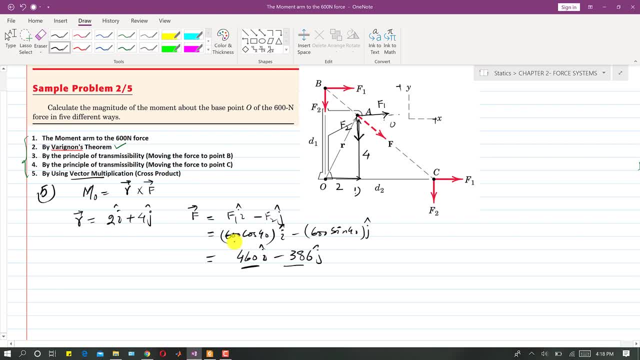 So now, if we take the cross product Of these two, So then what we will get To take cross product of this R and F, So we will write M about O. So this will be equal to i, j And k. 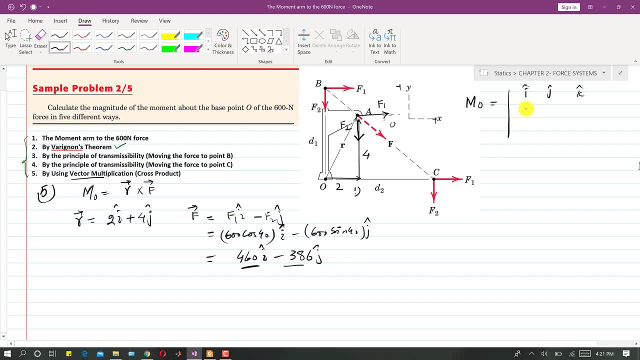 And I will write 2, 4.. And the k component of R is 0. Right, And this is 460.. Minus 386.. And the k component is 0. Right. So what we will do is that. 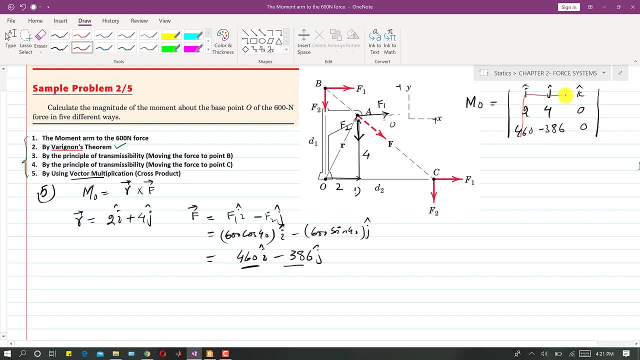 We will draw a line Right And then we will Find the determinant of this. So the determinant of this will be 0. So moment about O will be 0.. Into i Right? Then what we will do? We will draw another line on J.